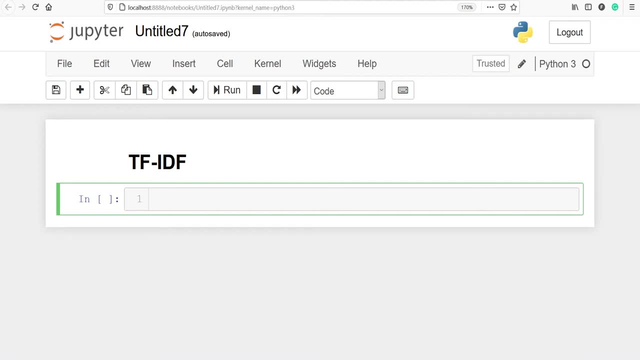 One way to represent word using frequency-based embedding is to use TF-IDF. TF stands for term frequency. IDF stands for inverse document frequency. In this video, you will learn about TF-IDF. TF-IDF is an improvement over count vectorization that we have already studied in. 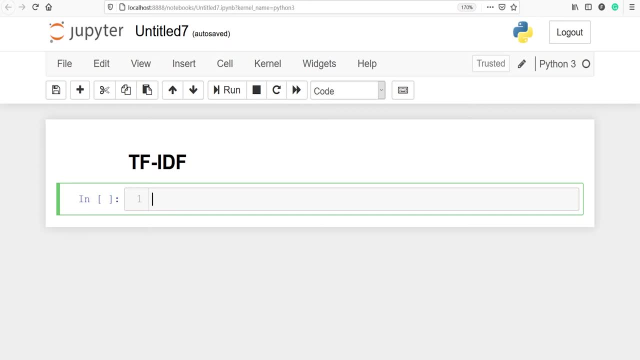 our last video on count vectorization. TF-IDF tries to capture how often a word occurs in a document, as well as how often that word occurs across the entire corpus. From sklearn. we will import the TF-ID vectorizer From sklearnfeatureExtractiontext: import TF-IDF vectorizer. 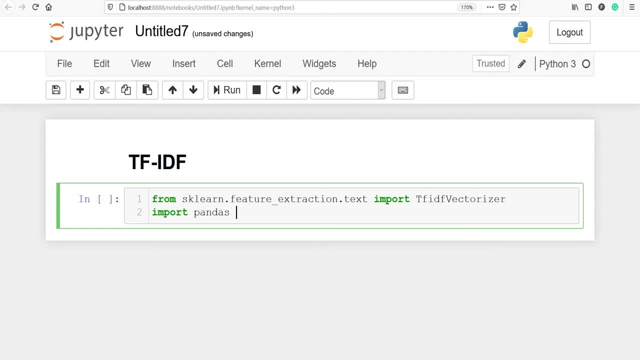 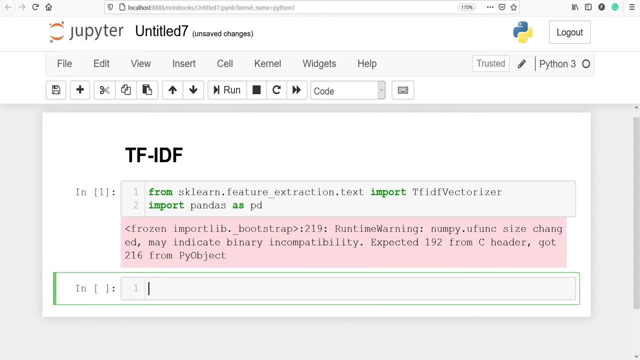 We will also import pandas speech. TF is a measure of how frequently the word occurs in some document. IDF is a measure of how infrequently a word occurs, the entire corpus, where the corpus represents all of the document that you are working with. Let's make a corpus. I will make one variable corpus. 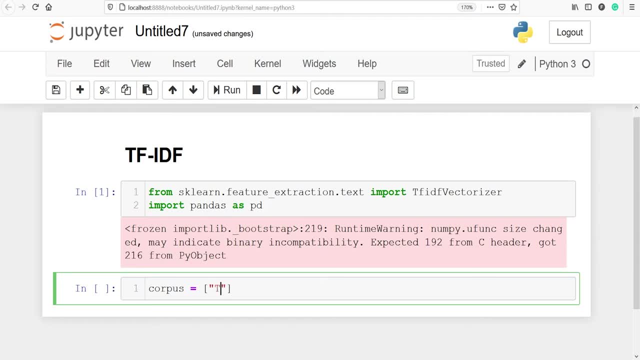 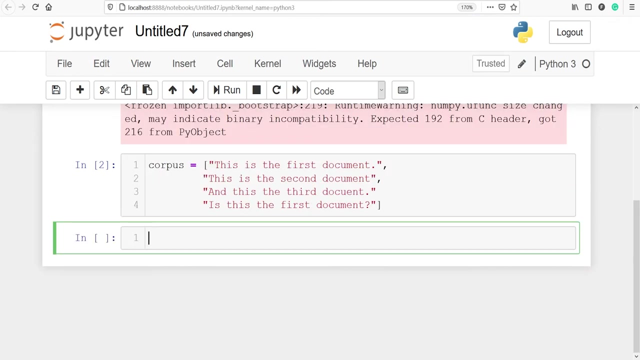 Inside this I will write some sentences. This is the first document, This is the second document And this is the third document. Is this the first document? Let's execute our code. Let's print a variable corpus, Print corpus. This is the entire corpus we got in the output. We can also look at the 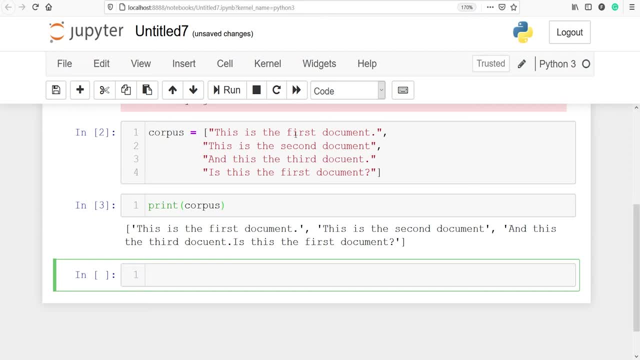 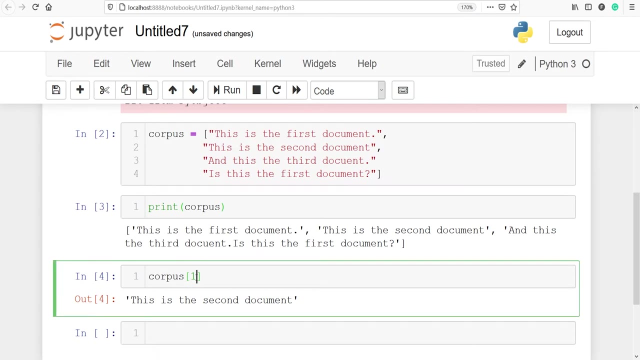 particular document. For example, we want to look at this first sentence. We can write corpus and index number One. So this we will get here. This is the second document To get this document. we will put zero here And in the output we will see we get. this is the first document. 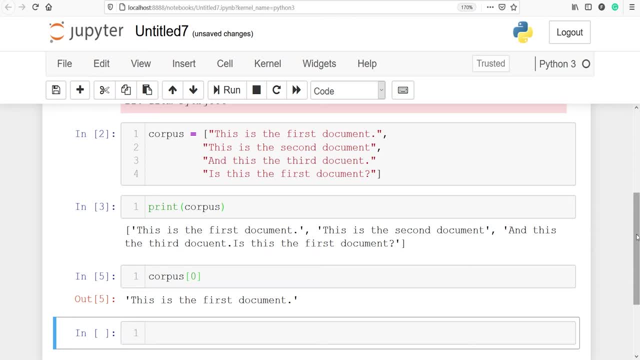 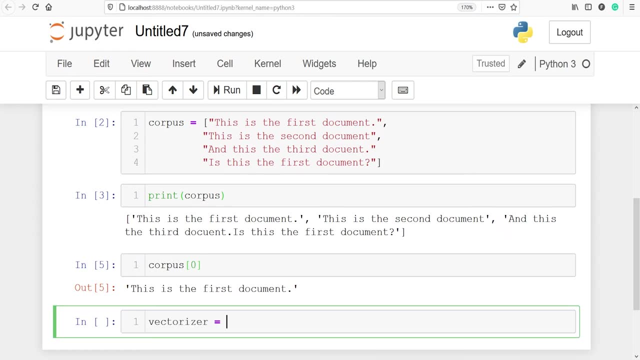 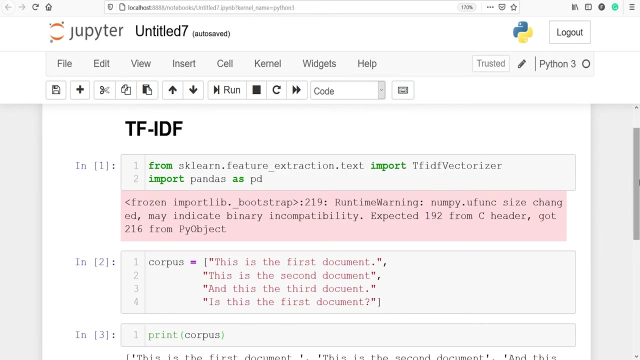 Let's instantiate the TF-ID vectorizer and save it in the object. I'll make the object vectorizer. Now I will call the class TF-IDF vectorizer which we have imported Here. and you can see, here we have imported the class TF-IDF vectorizer. Let's execute our code. 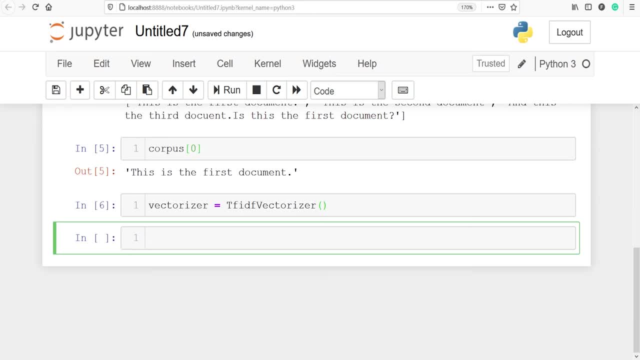 Let's fit it on the corpus and save it in a new variable. I'll make a new variable x. I'll call the object vectorizer. From this I will call the property fit, underscore transform. We are going to fit and transform on the corpus and save the result in the new variable x here. 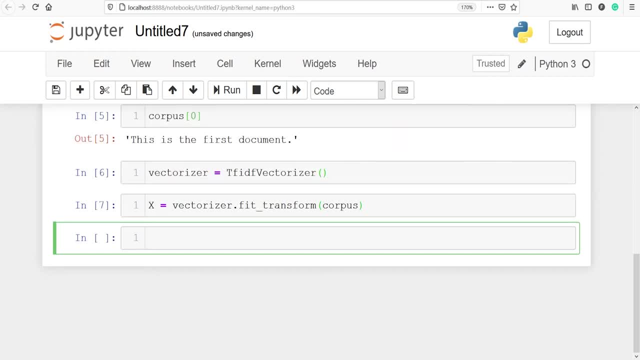 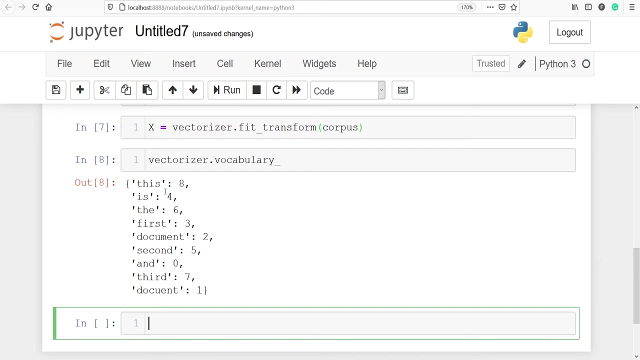 let's execute our code. next we will see the vocabulary. i will call the object vectorizer from this, i will call the property vocabulary- underscore. let's execute our code. and these are the vocabularies. and these numbers are the unique id associated with this vocabulary. let's count the. 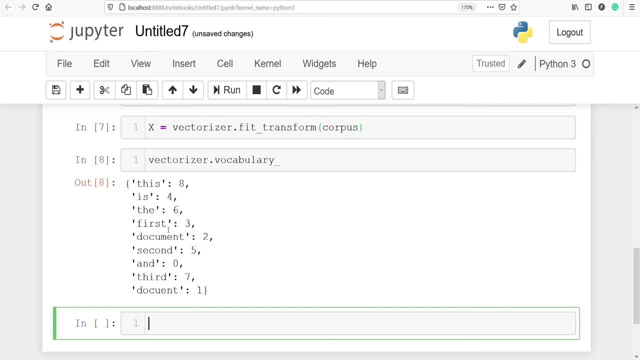 total number of vocabularies: 1, 2, 3, 4, 5, 6, 7, 8 and 9. we have 9 words here and the numbers are starting from 0 to 8, because all these words are unique. next we will find the feature names. 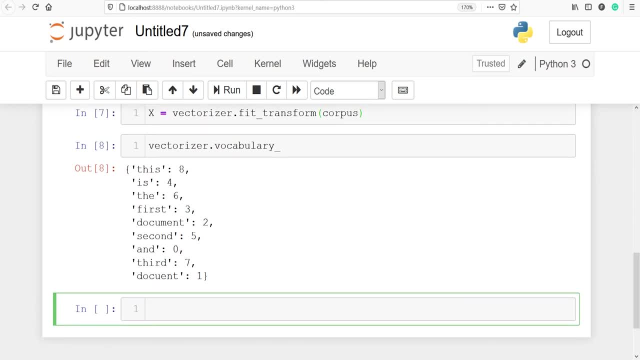 the vocabularies are the feature names. in real. i'll call the vectorizer from this. i will call the property get feature names. let's execute our code. in the output you can see we get the same number of vocabularies. we have 9 words here and the numbers are starting from 0 to 8. 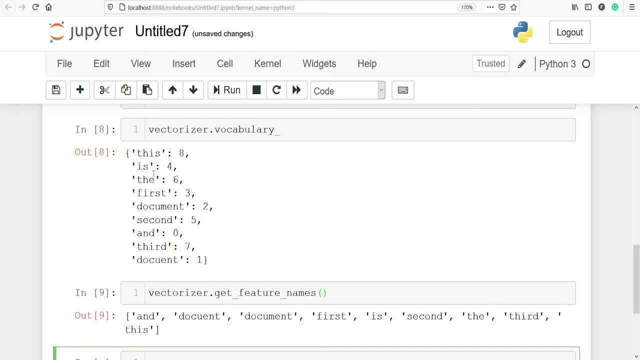 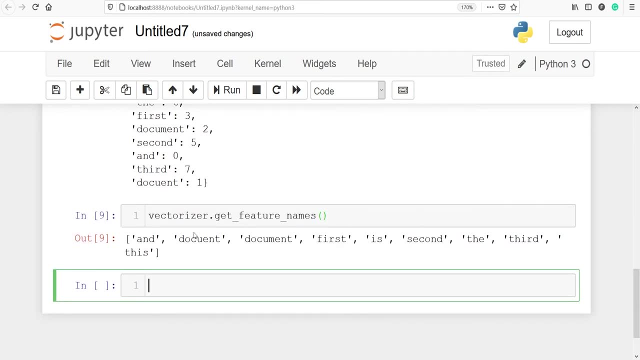 same words here. the only difference is here in vocabulary, because we get the words as well as the unique id, and in feature names we only get the words. here these are the features, or you can say the columns. let's see the idf score of features. we will see the idf score. we will call. 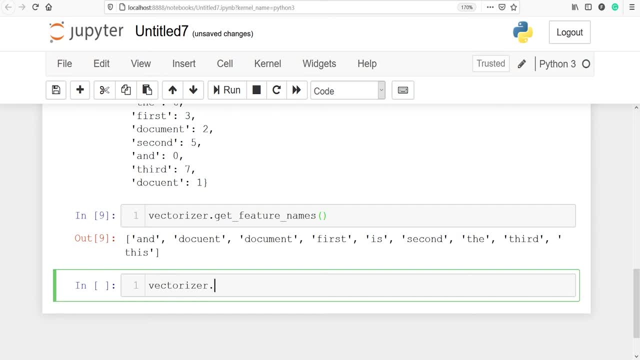 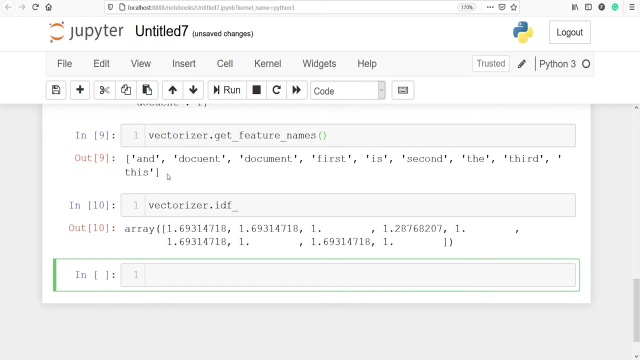 our object vectorizer and then we will call this idf underscore and these are the idf score of the object vectorizer and then we will call this idf underscore and these are the idf score of our features. here we have nine features: one, two, three, four, five, six, seven, eight and nine. 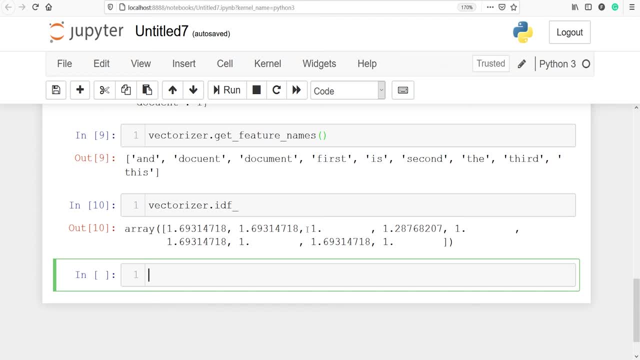 and here also we will get nine scores: one, two, three, four, five, six, seven, eight and nine. since we have nine features, we will get nine. idf score: the score one. this score one is the lowest score, because that word is repeating in all the document. and let's look at this word which 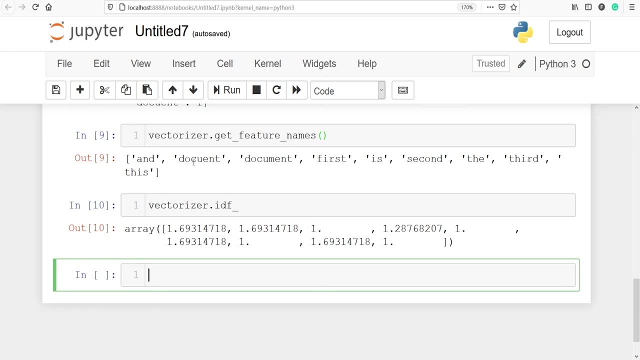 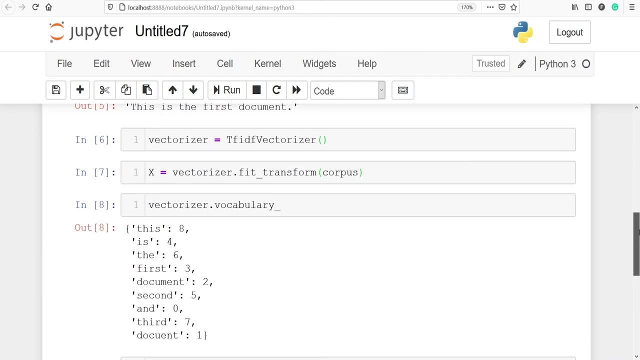 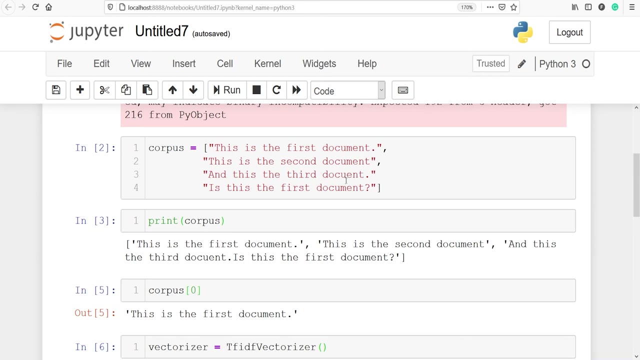 got the score one, one, two and three. one, two and three. this document is repeating everywhere and if we look at our here, you will see this word document is repeating everywhere. here i have made one spelling mistake, but now let's do not correct it, because we have already fit our model. 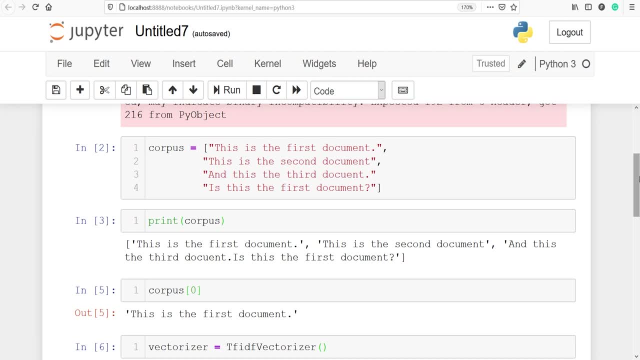 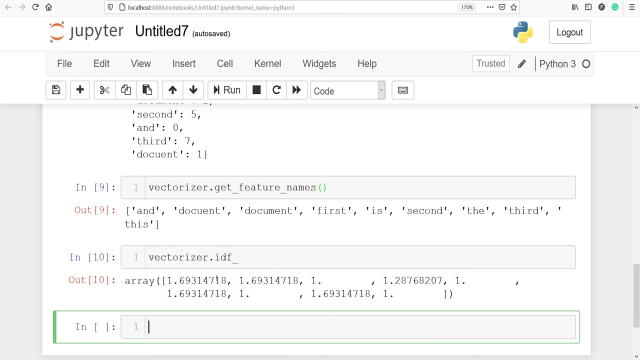 on this corpus. so, because this document is repeating again and again, we got the score of one, then here also we got the score of one. uh, let's find this one, one, two, three, four and five. one, two, three, four and five is is also repeating a lot of time, and here we'll see one, two and three is is. 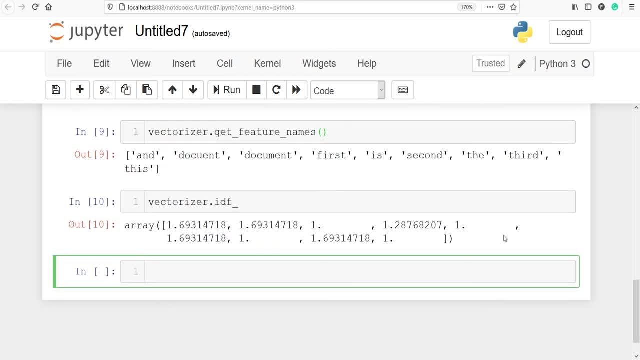 also repeating. that is why it got the score of one here. these are the scores here. one indicates the lowest score. the idf score will down the idf score and the idf score will go down. the idf score and the idf score will go down with those words that occur frequently across the entire corpus. 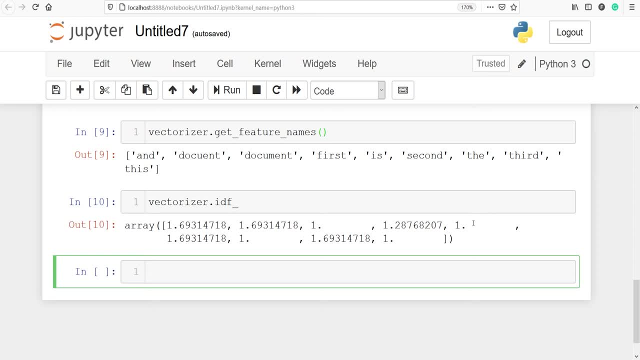 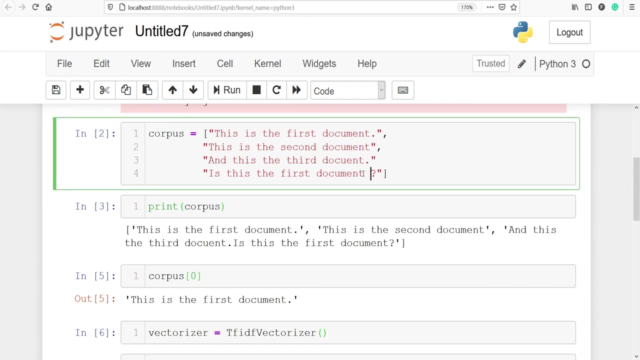 because these might be the common words, such as is a, the, he, she, etc. thus both tf and idf put together capture the significance of a word, a rare word that occurs very often in a particular document, as high, high weightage, for example. if i put one more word here, let's say i put 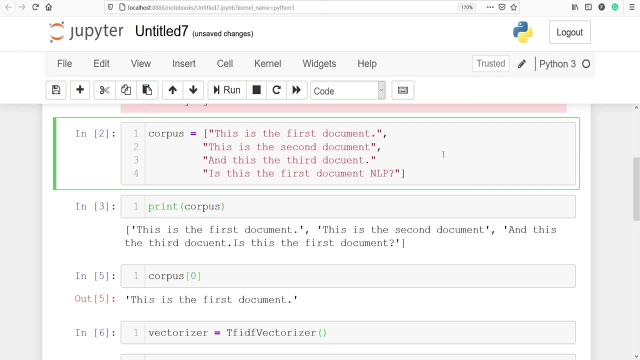 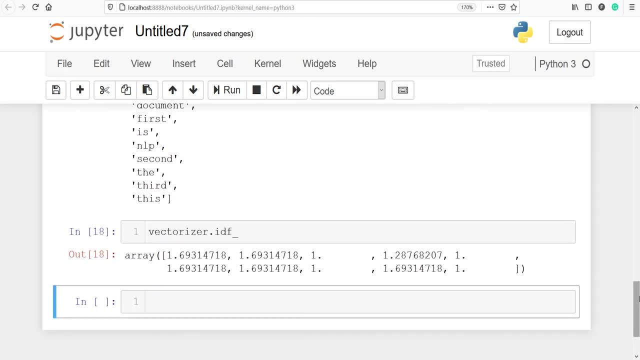 nlp and i'll run again and let's see if we see any changes in the score. and here you will see we are getting the same score, almost same score. we are not getting much changes here. let's make the document term matrix to get the scores of each feature. i'll make one variable document.